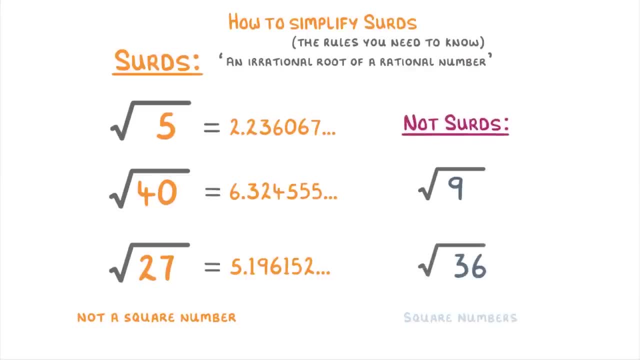 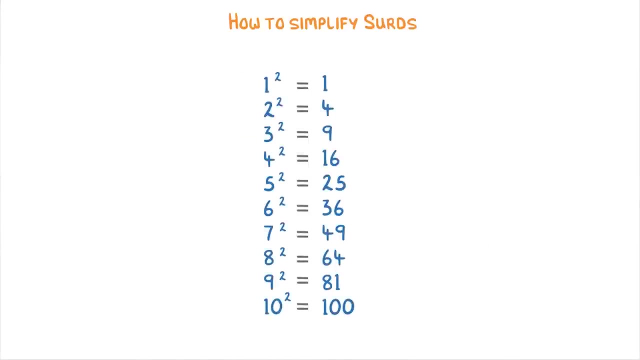 don't count as thirds, because 9 and 36 are both square numbers, with root 9 being 3, and root 36 being 6.. One thing that really helps with simplifying thirds is knowing all of your square numbers. So if you don't already know all of these, 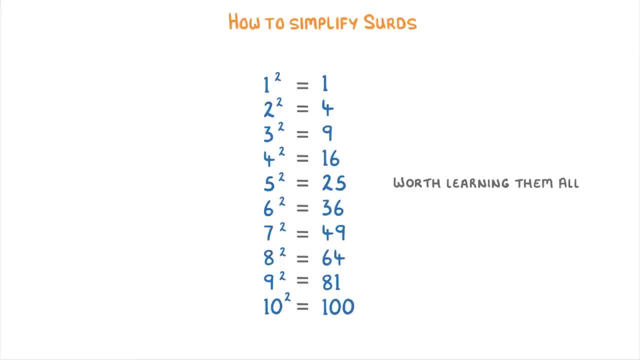 square numbers, then it's definitely worth learning them all before you try and do this topic. The other thing that you need to know before you can simplify, thirds, is how they multiply. If we took the square root of 3 and multiplied it by the square root of 5, then that's exactly the same thing as the square root. 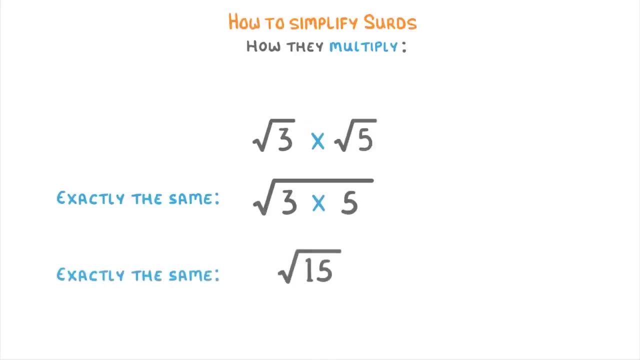 of 3 times 5, or the square root of 15.. This means that we can also go the opposite way and divide 1 third into 2.. For example, if we took root 40, we could rewrite it as a product of any of its factor. 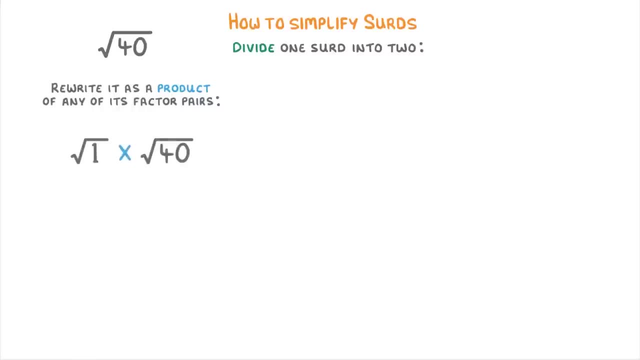 pairs, For example: root 1 times root 40,, root 2 times root 20,, root 4 times root 10, or root 5 times root 8.. One important point, though, is that this rule only works if you're. 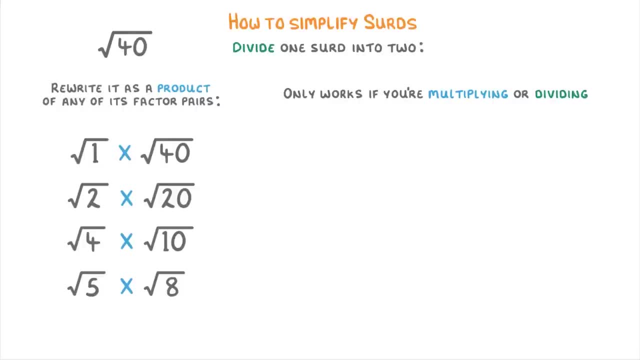 multiplying or dividing. So while you could rewrite root 40 as root 80 divided by root 2, because 40 equals 80 divided by 2, you can't write it as root 30 plus root 10, or root 60. 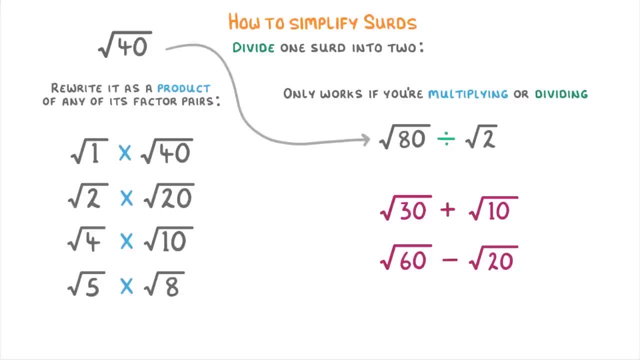 minus root 20.. Because even though 30 plus 10 and 60 minus 20 are both 40, we can only use this rule when we're multiplying or dividing, not when we're adding or subtracting. Getting back to writing them as the product of their factor pairs though the benefit. 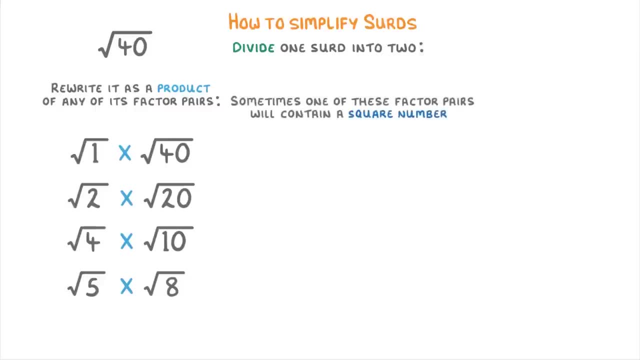 of doing this is that sometimes one of these factor pairs will contain a square number, like this one here, which has a root 4.. Because 4 is a square number, we can simplify the root 4 to a 2, so that it becomes 2 times root 10, which we write as 2 root 10.. So 2. 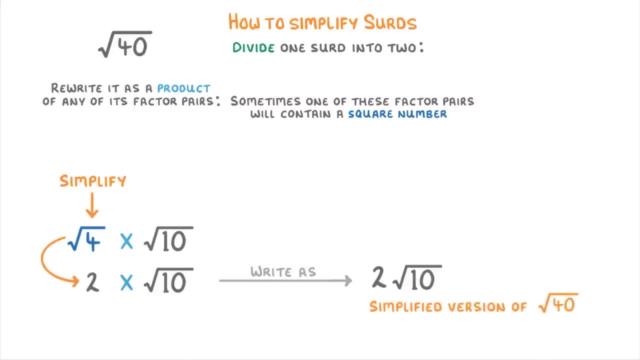 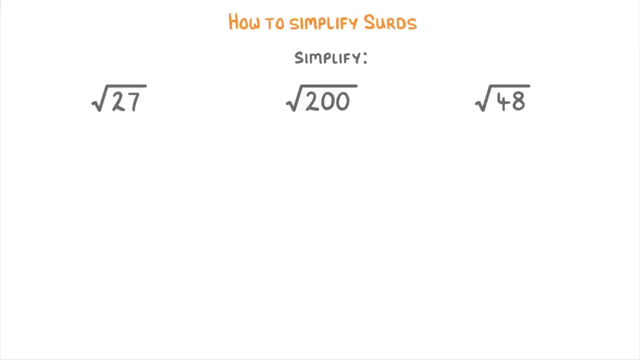 root 10 is the simplified version of square root 40. And that's all we need to do to simplify a third. Let's try the same thing for these thirds. So for the square root of 27, we need to find a factor pair of 27 that contains a square number. And if you don't just know it off. 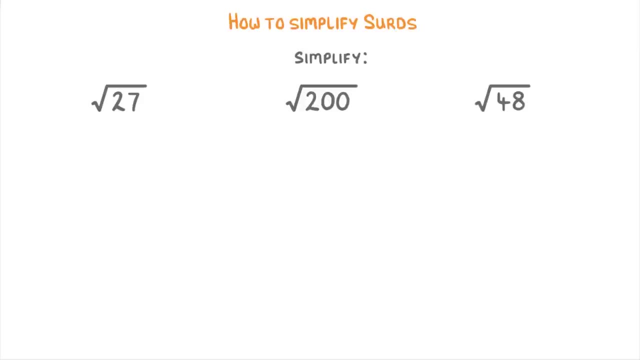 the top of your head you can write out all the factor pairs, So root 1 times root 27, and root 3 times root 9.. Root 1 times the original number is never going to help, though, so we can cross this. 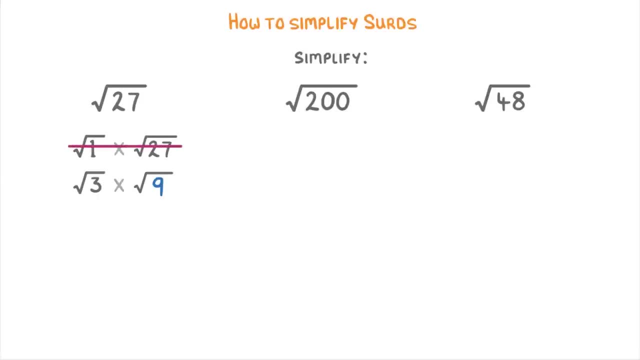 one out. The thing to spot is that the 9 here is a square number, So we can rewrite the root 9 as a 3, to get root 3 times 3.. Then swap them around to get 3 times root 3.. And then. 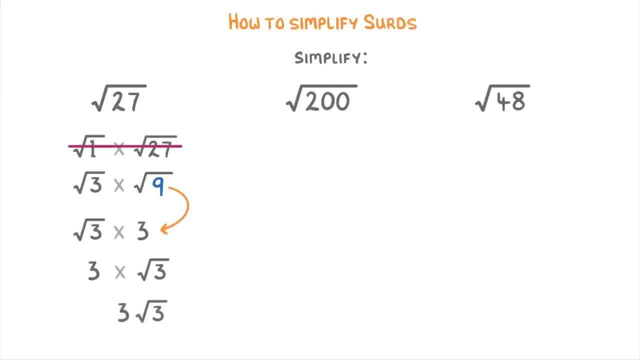 just write that as 3 root 3, as our final answer For the square root of 200, it would take ages to write out all the factor pairs, So you really just need to be able to notice that 100 is both a factor and a square number. 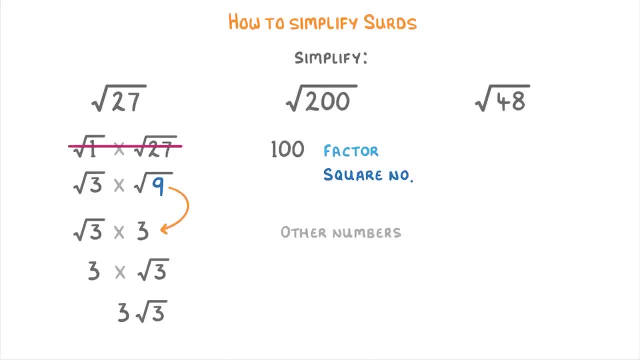 In this case. there are actually a whole bunch of other factors that are square numbers as well, like 4 and 25.. But, importantly, 100 is the biggest one, and you always want to go for the biggest square factor. You can still get the right answer if you pick a smaller. 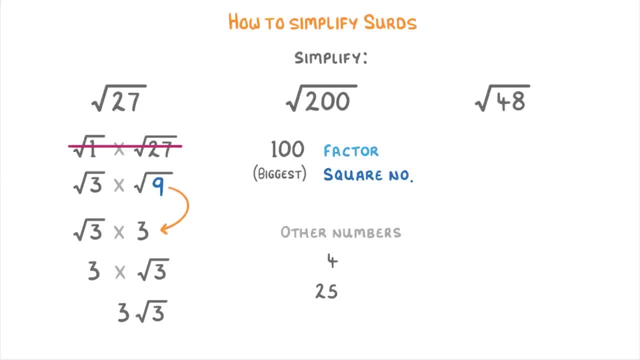 one, but you'll just have to do a few more steps. So if we go for 100, we'd have to times it by 2 to make 200.. So we can write out the square number and then just write out the number, and then just write out the number. to get the answer. So if we go for 100, we'd have to times it by 2 to make 200.. So we can rewrite out the number and then just write out the number, and then just write out the number and then just write out the number. 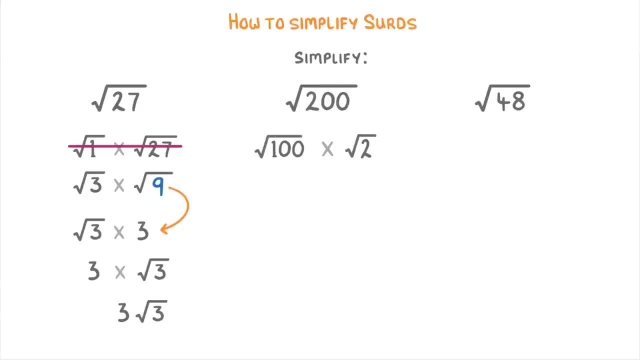 We could rewrite root 200 as root 100 times root 2,, which simplifies to 10 root 2, because the square root of 100 is 10.. For root 48, the easiest way to do it is notice that it's equal to root 16 times root 3,, which 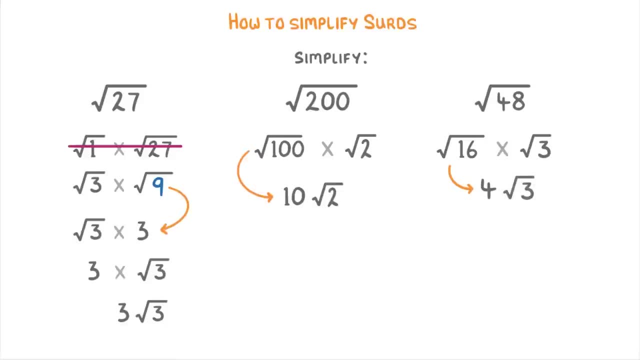 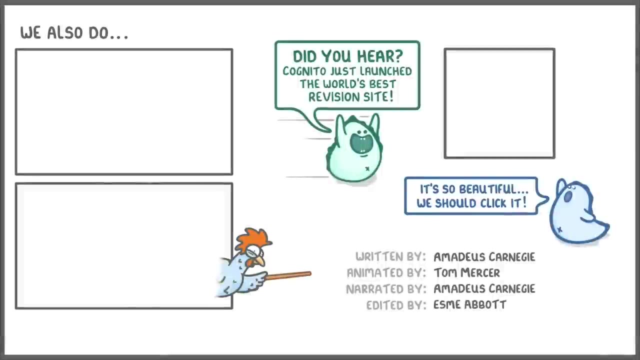 we can simplify to 4 times root 3, or just 4 root 3.. Anyway, that's everything for this video, so hope you found it useful. if you did, then please do give us a like and subscribe, and cheers for watching. 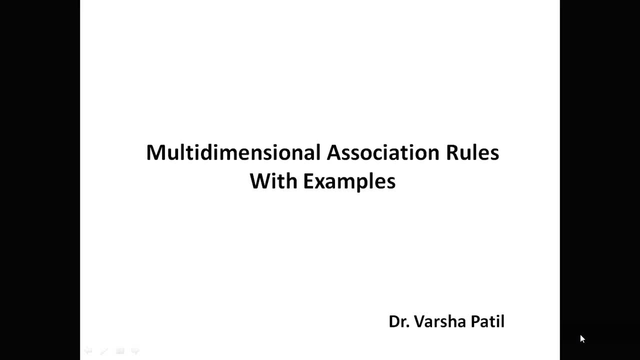 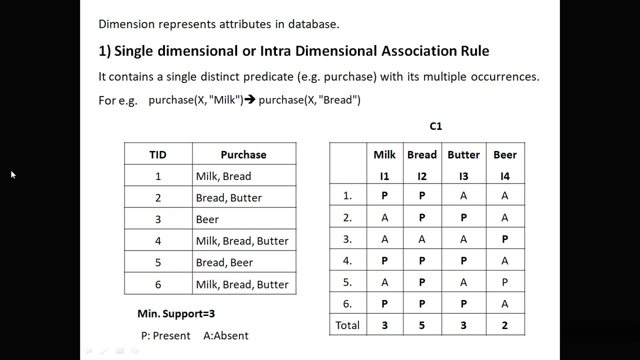 Dear listener, welcome to my channel. Topic of this video is multidimensional association rule. In this video I am going to explain how to generate multidimensional association rule with the help of a priori algorithm. Dimension represents attributes in database First type: single dimensional or interdimensional association rule. It contains single distinct 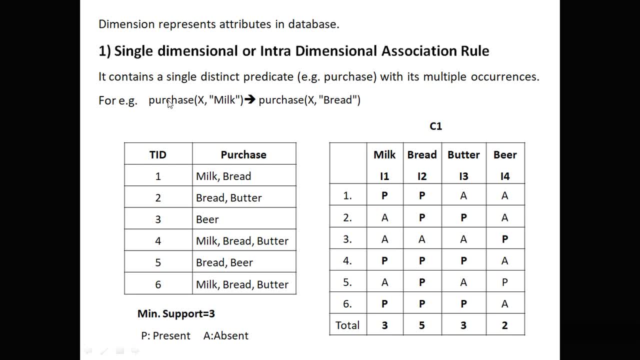 predicate with its multiple occurrences. For example, purchase is a predicate here. that milk implies bread Rule is written like: purchase x milk implies purchase x bread. Now here purchase is repeated, that is, with its multiple occurrences. This is the rule with the two item set. If three item sets are there, then purchase. 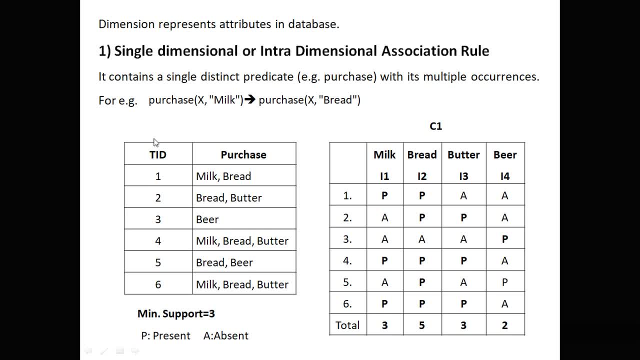 comes with and operator. Now see how to generate such a type of rule. Take an example: six transactions are there, 1 to 6, and in each transaction represents the purchase of that particular item. Minimum support 3 is given. Now we require to convert this table into: 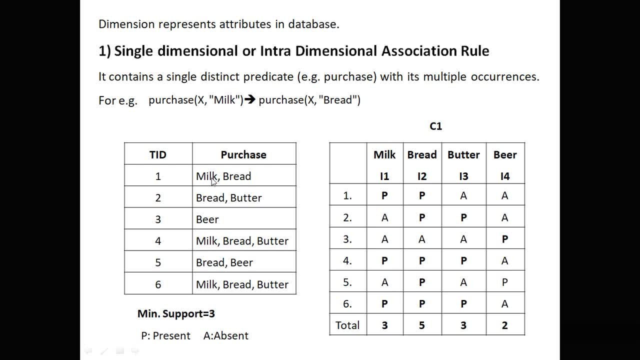 different format. Now we are giving for milk as item i1, for bread i2, for butter i3 and for beer i4.. So for items i2 and i3, we are giving for milk as item i1, for bread i2, for butter i3, and for beer i4. 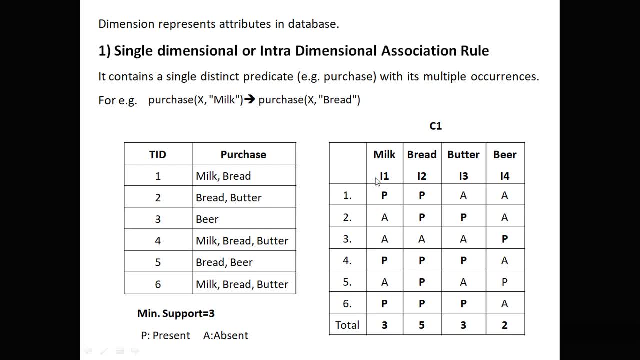 So for items i2 and i3, we are giving for milk as item i1, for bread i2,, for butter i3,, for butter i3, and for beer i4.. now first we write: milk and bread is present, so pp is only for i1 and i2, that is milk and bread. 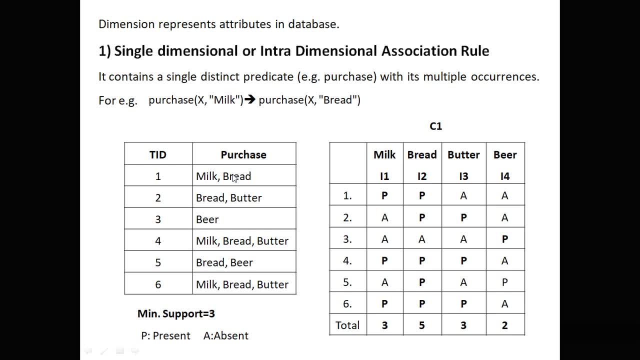 and for other it is aa. so in this way we require to convert this table into this table in the format and that table we can name as candidate set 1, that is c1. now here we make the addition of p elements at the column level which represents the support count for that particular item. now